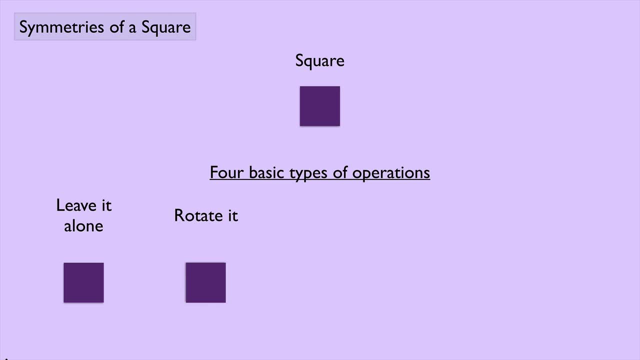 We could also rotate the square. That would bring the square back to where it was. We could also flip it about a perpendicular bisector. So what I mean by that is we would flip it. 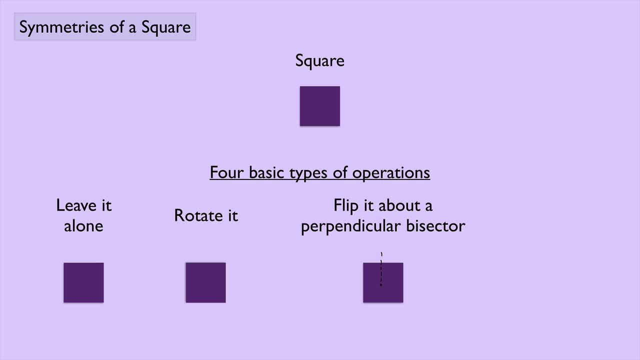 We could flip it maybe around this axis right here. This would be like a perpendicular bisector, so that would be flipping it around there, or another perpendicular bisector would be right there. This would be another place that we could flip it about, or we could flip it about a diagonal, and there's two ways to do that. Because there are two diagonals, we could flip it about that diagonal, or we could flip it about this diagonal. 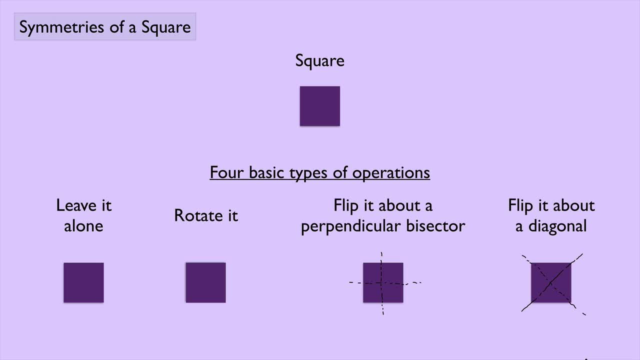 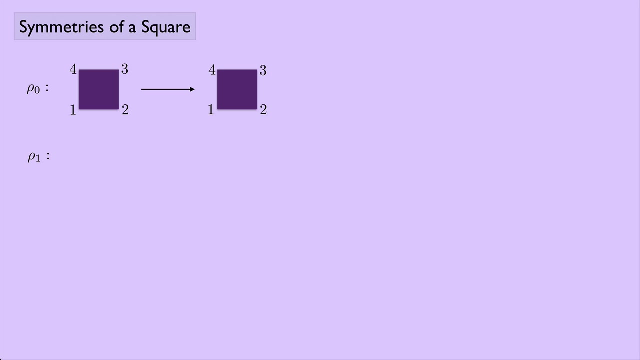 So we're going to look at each of these four types of operations. So the first operation, I'm going to call that row with a subscript zero, and that's the one where we take the square and we leave it alone. So I'm going to number the corners of the square, one, two, three, and four, and this is going to make the square stay exactly where it was, one, two, three, four. Next, I'm going to have row with a subscript one, and think of row as rotation, just as we did with the triangle. 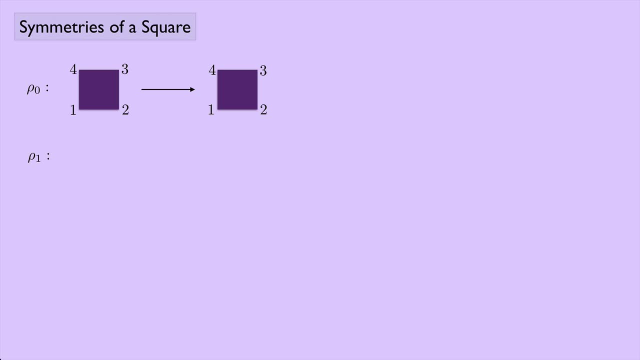 So in this case, I'm going to rotate the square counterclockwise. 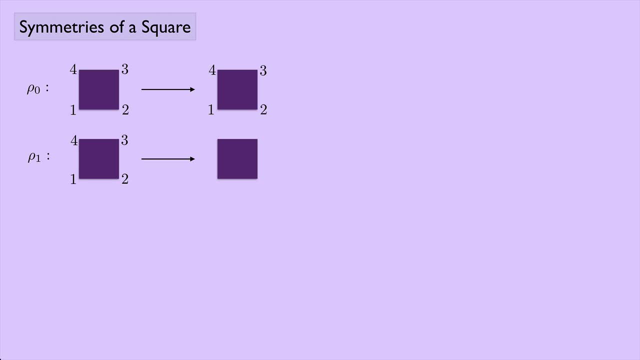 So here's the square I'm going to start out with, and it's going to become something that looks like this. 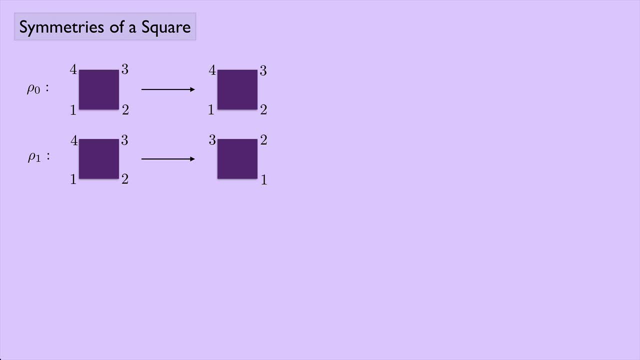 So the one now is going to rotate over here, the two will be up here, the three over here, and the four down there. 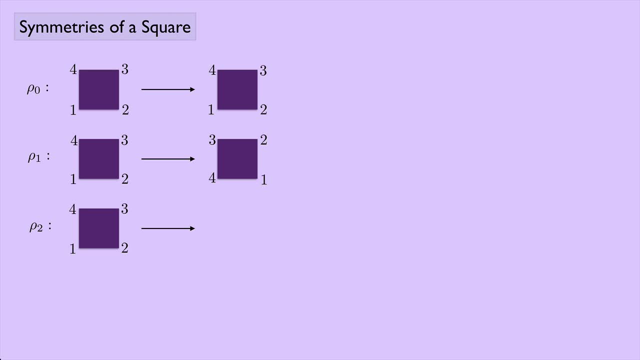 Next, I have row two, and that's going to take the square, and it's going to rotate it twice, in a sense, back to where the square was. So now, the one is going to be up here. The two here. The three here. And the four here. 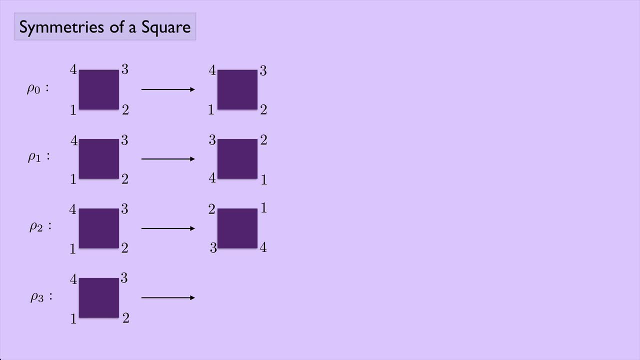 Then I have row three, and that's rotating the square one more time. So now, the one will be over here, the two here, the three here, and the four here. 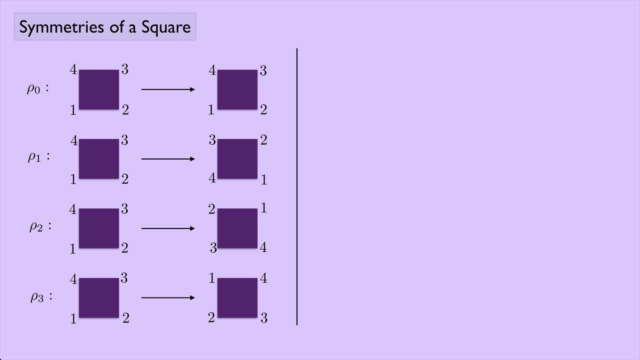 Alright, that takes care of the leave it alone and the rotate it types of operations. 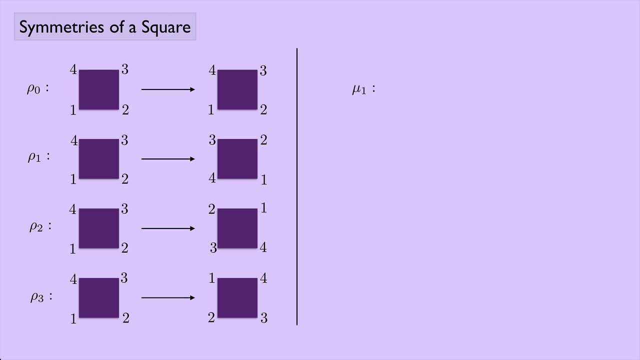 What about flipping about a perpendicular bisector? So for that, I'm going to call this mu with a subscript one. Here's my square. And what I'm going to do is I'm going to flip it about a perpendicular bisector that goes straight down the middle. So the bisector that I'm looking at is this one right here. So if I look at this axis here, it looks like the one and the two are going to switch places, and the three and the four are going to switch places. So now, the one will be over here and the two over here, and then the three will be here and the four over here. And then mu two would be a flip about the other perpendicular bisector. 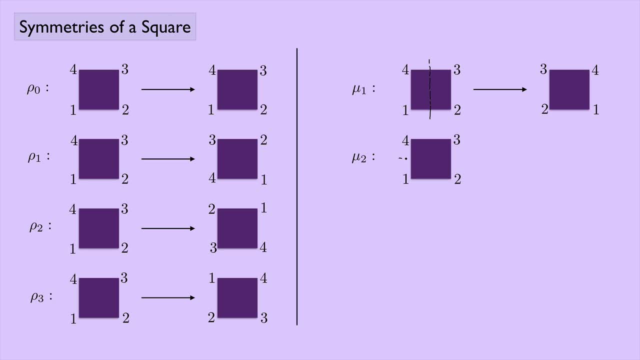 So now, that's going to be flipping about this bisector right here. And so, it looks like if I were to do that, that the one and four will switch places and the two and the three. So the one will be here, the two will be up here, the three down here, and the four down here. 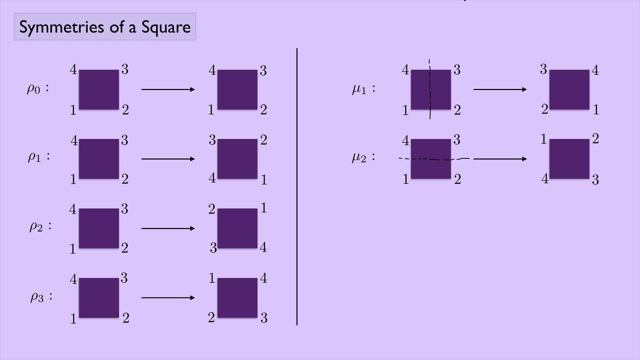 And now, I want to look at the last basic operation. That was flipping about the other perpendicular bisector. 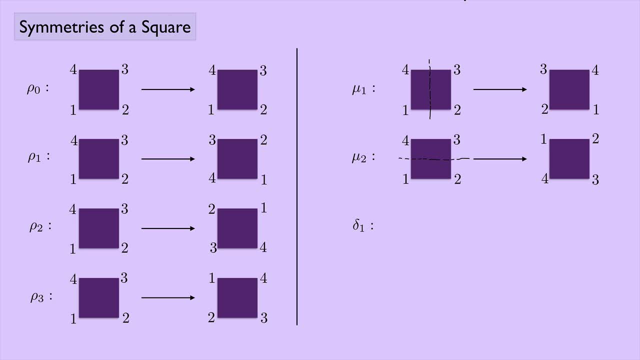 And for the diagonal, I'm going to use delta. And this will be a delta subscript one. So that's going to flip about this diagonal right here, the one going from the four down to the two. So the two and the four shouldn't change places. They should stay where they are. 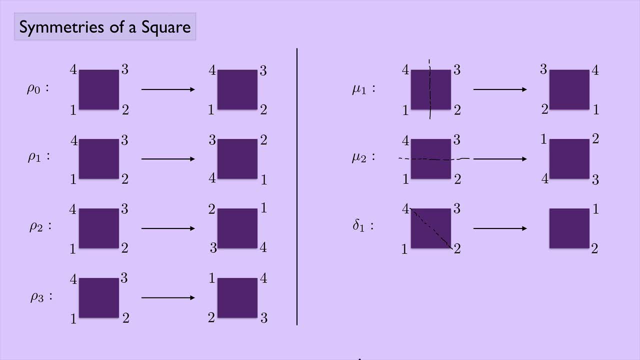 The one and the three should swap. So the one will be up here, the two will stay where it was, the three will be down here, and the four will stay where it was. 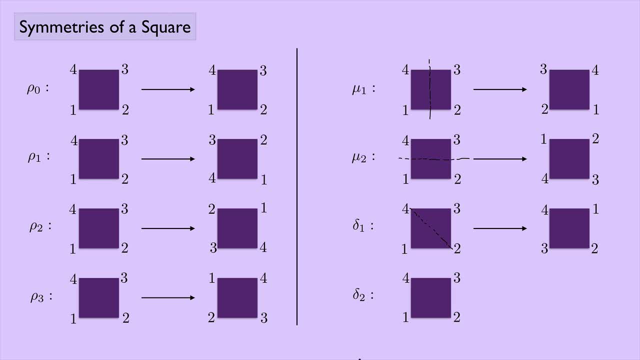 And then the last one, delta two. That will be a flip about the other diagonal. That's the one that's joining the one and the three. 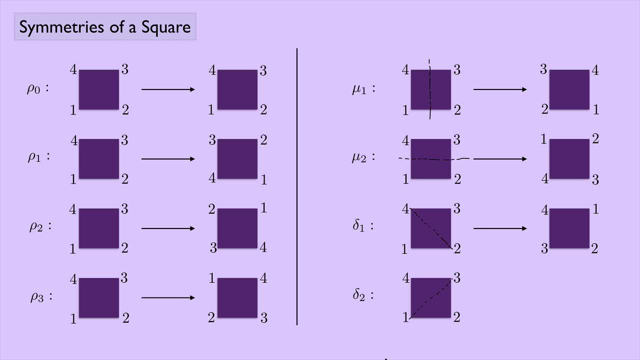 So that's this diagonal right here. So the one and the three should stay where they are, and the two and the four should switch places. 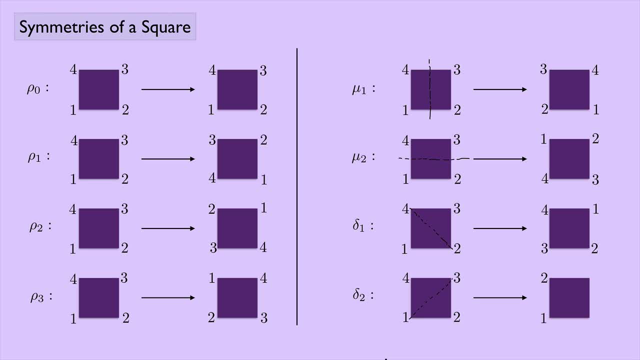 So the one will stay where it was, the two will be up here now, the three will stay where it was, and the four will be down here. 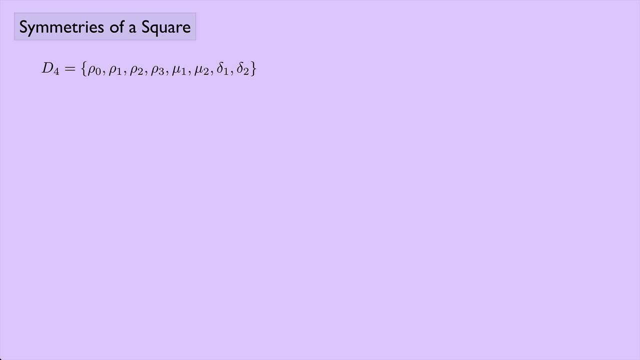 So these eight operations form a group. And I'm going to call that group D with a subscript four. And it has eight elements. And you should know that the naming of this group, this D4, is not unique. Some people call this D8. This is a dihedral group. Any of the symmetries of a regular polygon will be labeled with a D for dihedral and then a subscript. And so you should know that I am calling this D4, but some textbooks would call this D8 because it has eight elements. I'm calling it D4 because it has four sides. 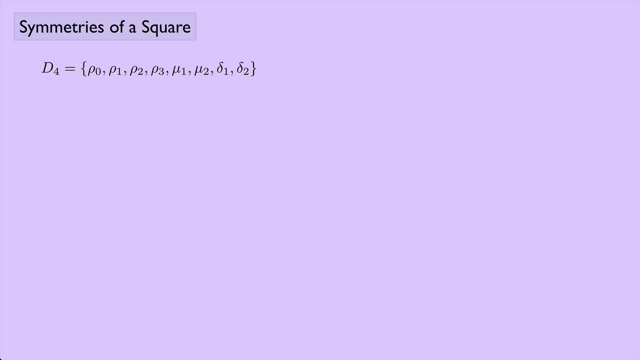 So in this case, we have eight operations. And the binary operation, just as it was before with the triangle, is composition of functions. And we can think of each of these operations here, each of these elements of the group, as a function from the set one, two, three, four to the set one, two, three, four. So let's look at an example. Suppose I look at delta one. That was a flip about the diagonal that was joining two and four. Well, if I look at the two sets, one, two, three, and four here, what happened? Well, the one that went to a three, the two stayed where it was, the three went to one, and the four stayed where it was. So you can see how each of these elements of this group really is a function on the set one, two, three, and four. 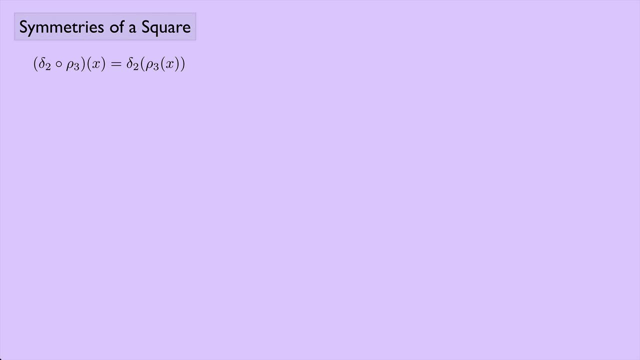 So if that's the case, then we should be able to compute something like delta two composed with row three. This is composition of functions. So it's delta two of row three of x. So here's row three. That's the thing that did the rotation. And delta two, that was the thing that flipped about the diagonal that joined one and three. But remember, composition of functions acts in a certain order. So the first thing that we would do is this row three. That's the inside part. 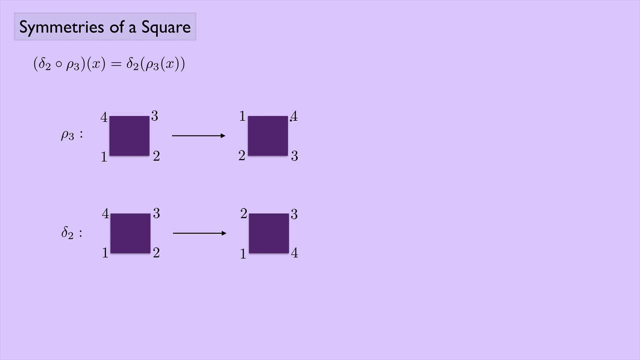 And then delta two is going to act on this square right here. So what did delta two do? Well, that was the flip about this diagonal. So this thing here and this thing here stay the same, and these two swap. So these guys here, they swap. But remember, we're acting on this square right here. So this isn't really a four. This is really a one. This isn't really a one. This is really a two. This is not really a two. This is a three. And this is not really a three. This is a four. I'm just copying the numbers that are on this square right here. 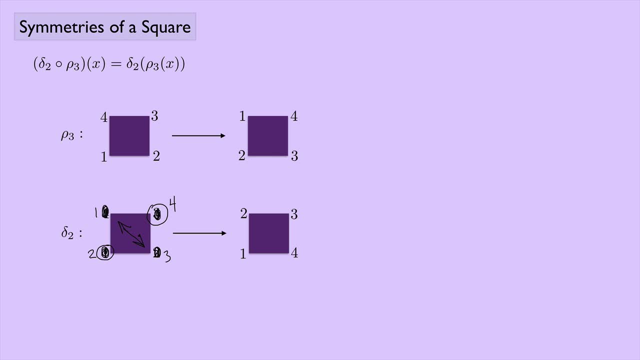 I'm bringing them down here. And so these two are going to swap places. 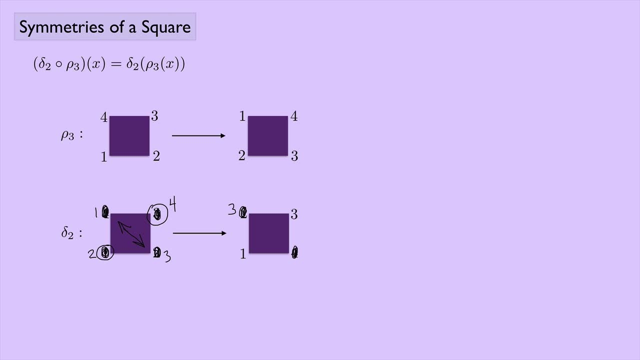 So the three will be up here, and the one will be down here. 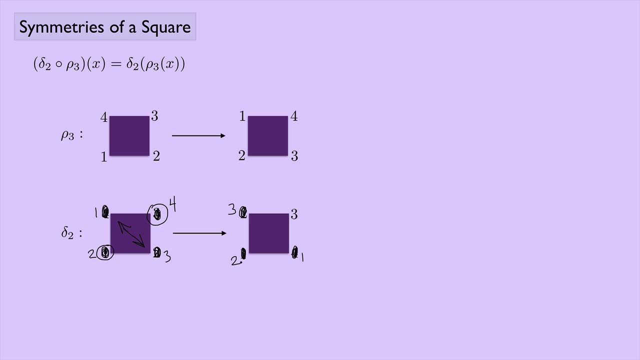 And these two are going to stay where they were. So the two will stay here, and the four will stay here. If we look at this in terms of our functions on the set one, two, three, and four, it looks like one, which initially started up here, switched to be down here. So what did that do? Well, the one went where the two was. So the two, if you look where we started here, the two was here. So the one went where the two was here. What happened to the two? So the two, which is here, swapped places with the one because it ended up down here. 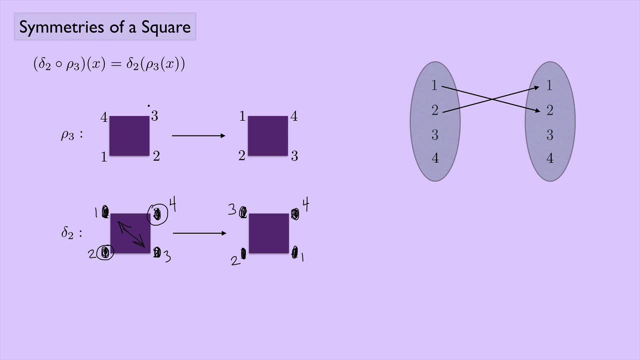 And then what about the three? The three, which was right here, now is over here. And so that swapped places with the four. And so the four went to where the three was. So this looks a lot like mu one. Mu one does exactly this. So we can say that delta two composed with rho three is mu one. 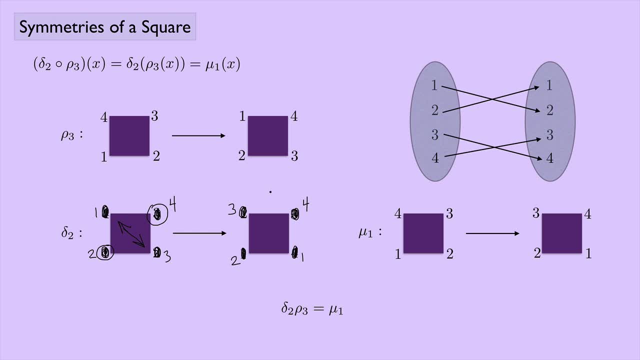 Or in shorthand, delta two rho three equals mu one. 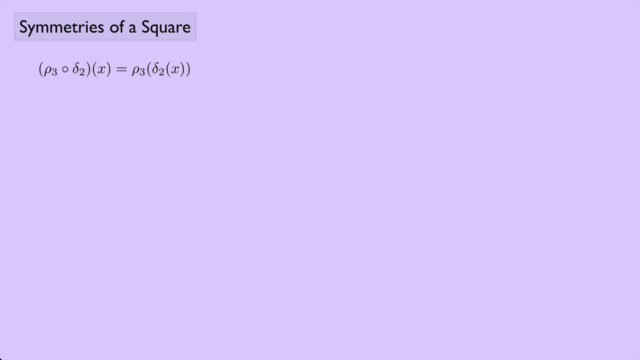 Okay, now let's look at rho three composed with delta two. 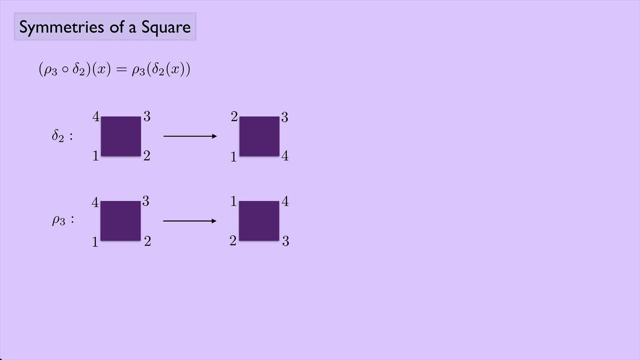 So here's delta two, and here's rho three. And remember what rho three does. Rho three is a counterclockwise function. Rho three is a counterclockwise rotation all the way around so the one then ends up all the way up here. So another way to think of that is to think of it kind of going back in this direction. It would be accomplishing the same thing if everything just went back one space clockwise. Okay, but remember, this is not the square that we're acting on. We're acting on this square, actually, for composition of functions. So the one actually stays where it is. 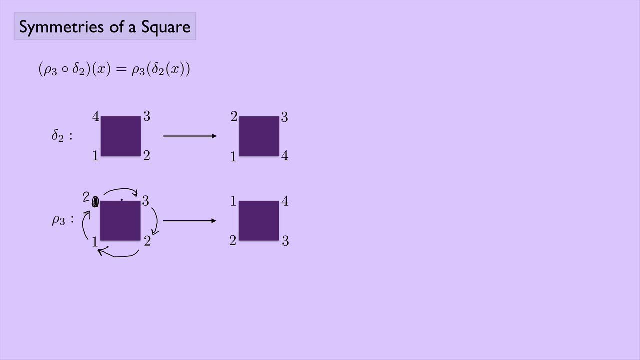 This four is actually a two. This three stays where it is. And this two is actually a four. And now I have to rotate everything. So this one is now up here. Well, that's perfect. There it is. This two is now over here. So that's really a two. This three is now down here. 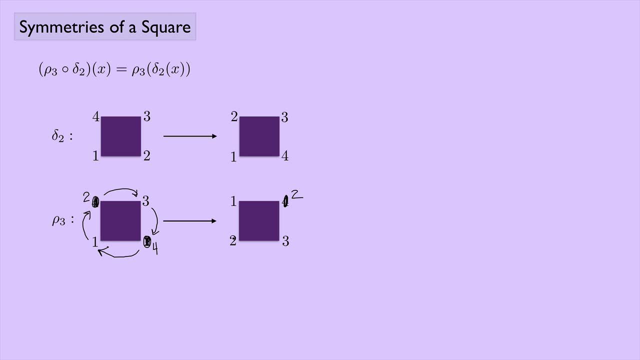 Perfect. There it is. And this four is now over here. So this is actually a four. 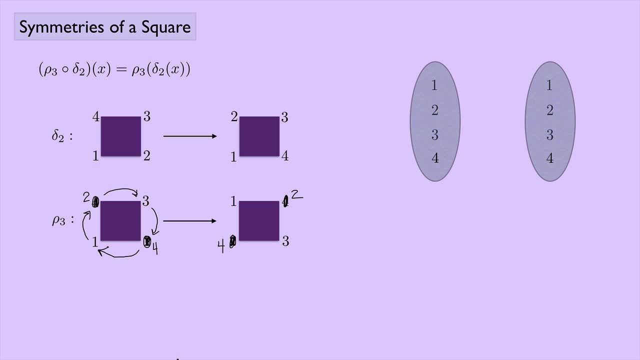 And now let's look at this on the sets one, two, three, and four. What happened to the one? So the one, which was right here, ended up up here. 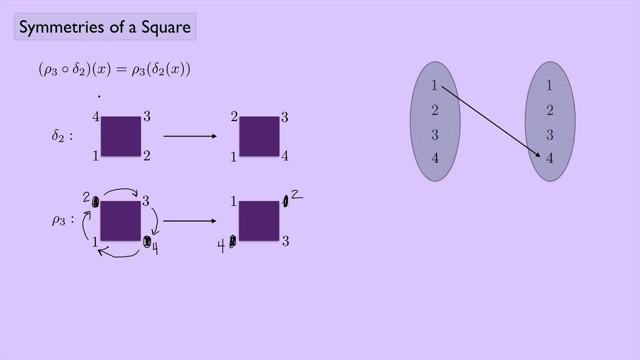 So it kind of swapped with the four. So the one went to where the four was. How about the two? Well, the two, which was down here, ended up up here. 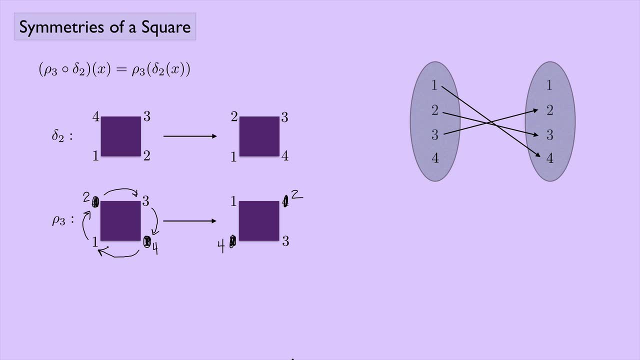 The two swapped with the three. And then the three swapped with the two. And the four swapped with the one. This looks a lot like mu two. So we can say that row three composed with delta two is mu two. 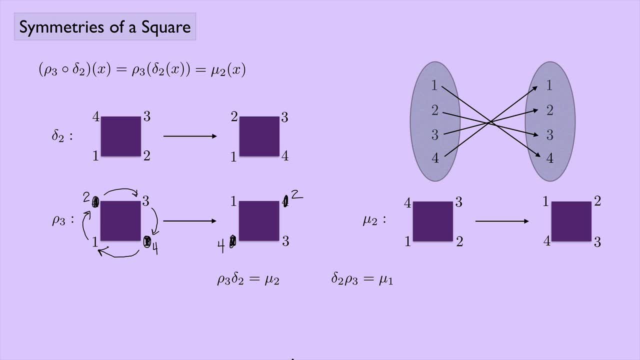 And so we also saw from before that delta two composed with row three was mu one. So in particular, row three delta two does not equal delta two row three. 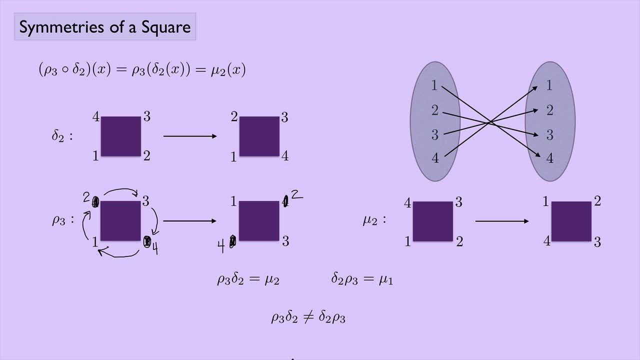 And this is a non-abelian group. Order matters. 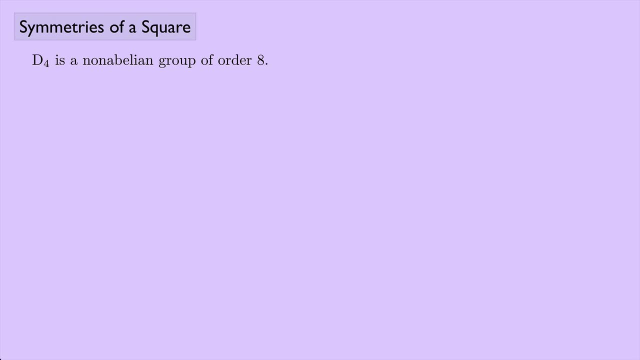 So now we see that D four is a non-abelian group of order eight. So let's look at the group table. So for this table here, we're going to list the eight elements that we have along the top here. So we have row zero, row one, row two, row three. And then we have our mu one and mu two. And then our delta one and delta two. 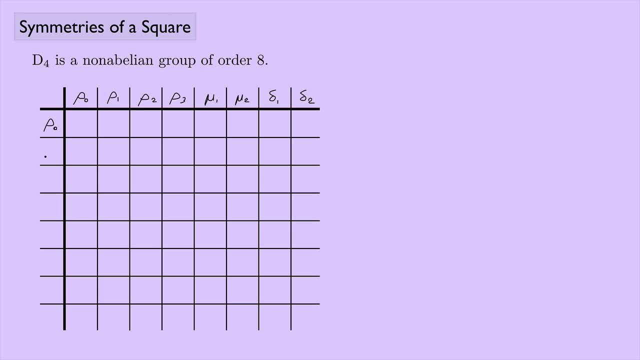 And then same thing along the side here. So we have row zero, row one, row two, row three. And then we have our mu one, our mu two, our delta one, and our delta two. And the order that we're going to compute in, first we're going to do something from the left 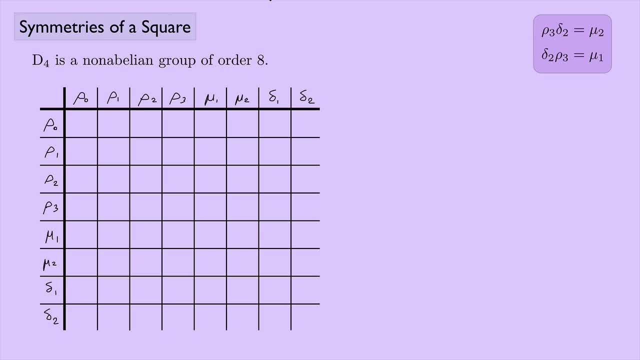 and then on the top here. So if we look at what we had before, we had row three delta two equals mu two. 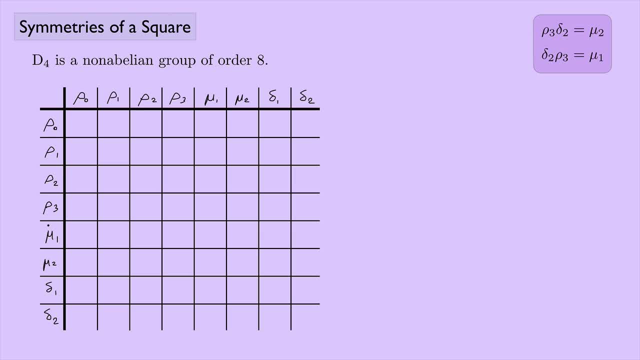 That means the row three I'm going to look at on the left here. So this row three right here. And then we'll go to the delta two. And then this spot right here should be mu two. And then we also saw that delta two row three, so here's delta two, here's row three, that was mu one. Okay, so I can fill those two in right now. 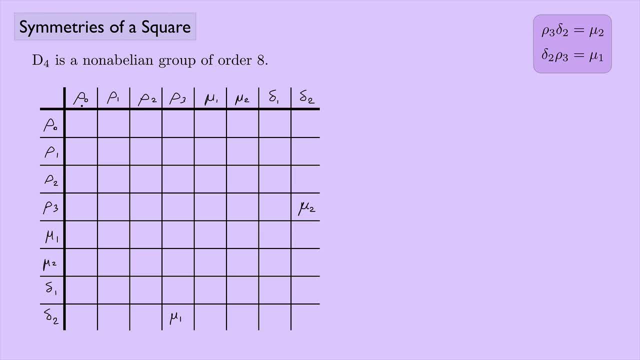 What else can I fill in? Well, I know that row zero didn't do anything. I just left it alone. So that means I can just copy this row right here. Everything can just come down here. And then, similarly, this column right here I can copy. So this is row one, row two, same thing all the way down. 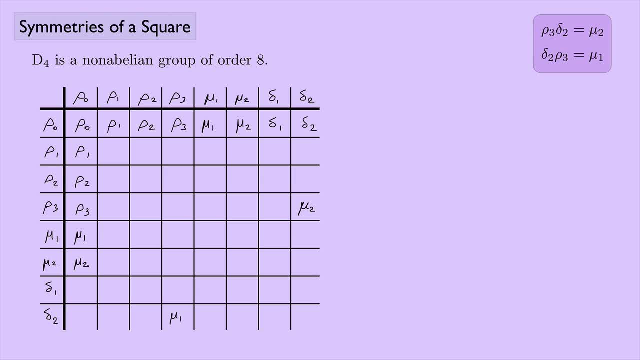 And by the way, these letters I'm using to denote these operations are not unique. There's different notations. This is just the notation that I happen to be using. Different textbooks will maybe call these different things. But this is what I find to be helpful. Now what about row one and row one? Row one composed with row one. 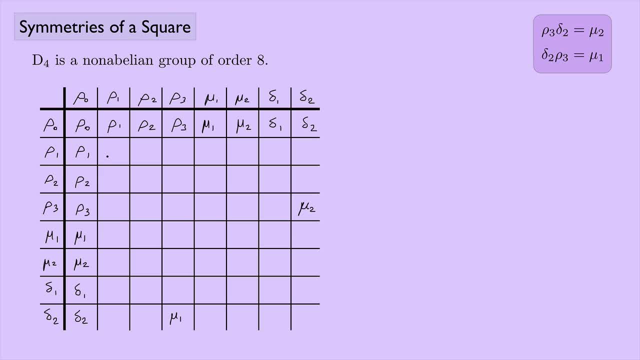 So that should be, if you imagine doing two rotations, that should be the same thing as row two. 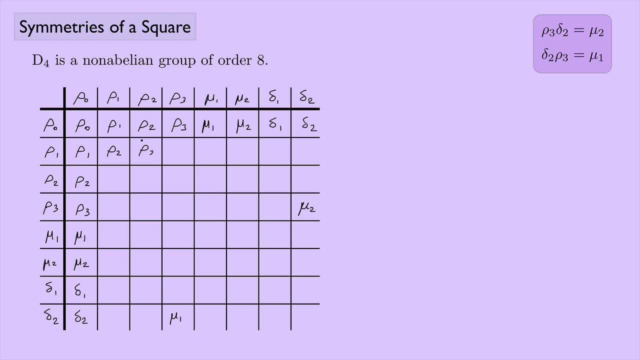 Row one and row two should be row three. And row one and row three would bring us back to where we were, that would be row zero. Row two and row one, that should be row three. 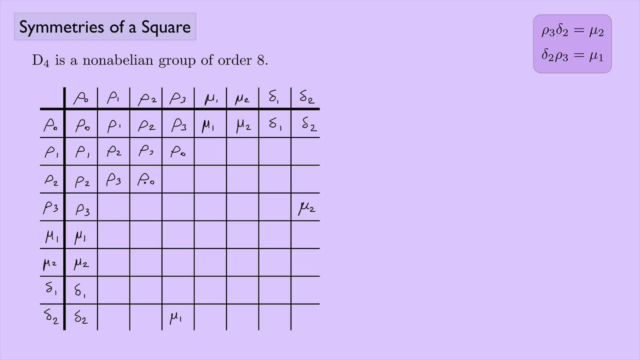 Row two and row two, that should bring us back to where we were. 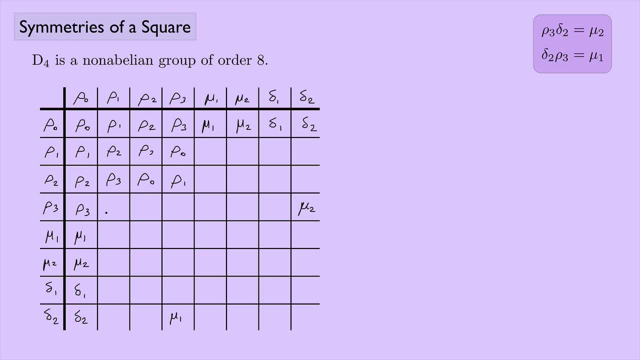 And row two and row three should bring us to row one. And so you kinda see a pattern here. 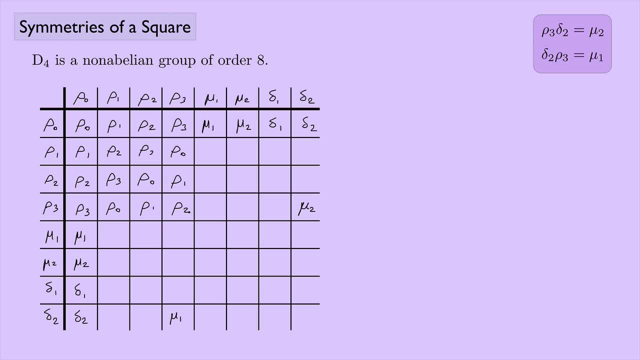 This'll be row zero, this'll be row one, and this'll be row two. Okay. What about the flips? 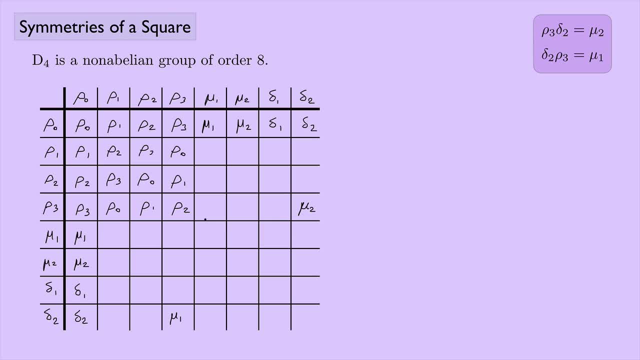 about the flips? Well, if I were to do mu 1 and mu 1, that would kind of undo one another, so that should be row 0, and that should be the same for any of these flips here. This should always give 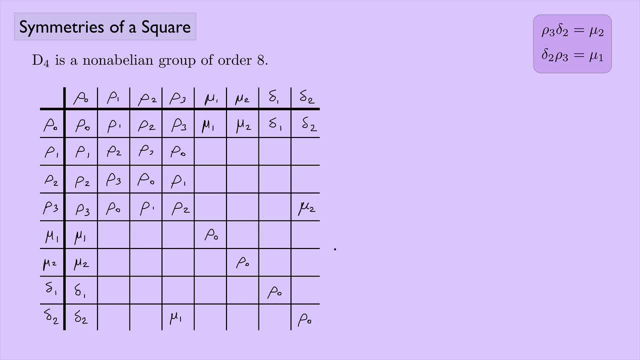 us back row 0 for all of these. Okay, so now comes the part where we have to do some computations, 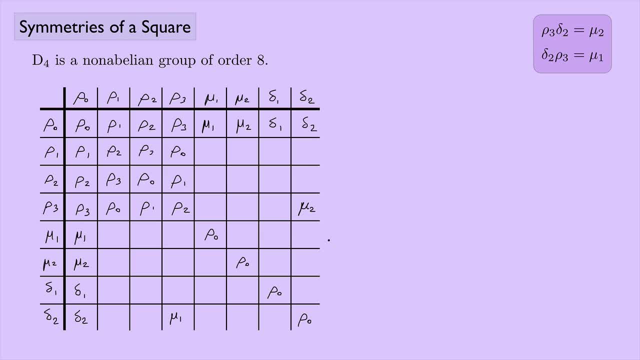 and so I'll leave you to figure out exactly why these happen to be what they are, but I'll just 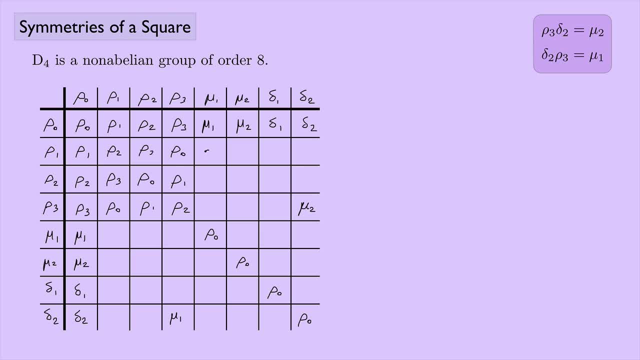 fill in a few of these here so we can get the idea. So this is a delta 1, and this is a delta 2, 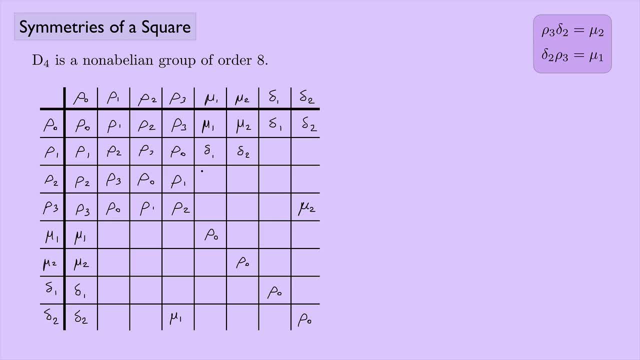 and remember the other rules that in any row or any column, each element should appear exactly once, so that's another way that we can kind of figure out what's going on. So now this right here, I'll tell you, is a mu 2, which means this has to be a mu 1 right here, just has to be. 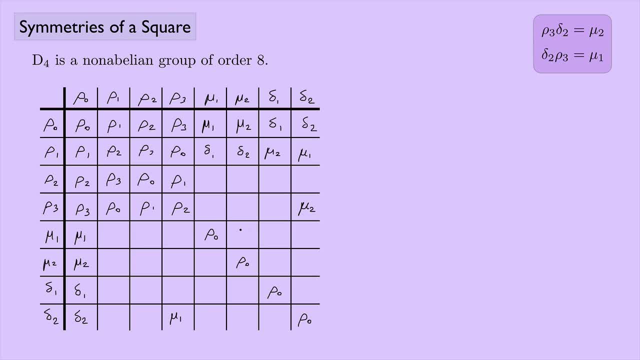 I will also tell you that this square down here, a 4 by 4 square, will be all rows, which means that this must be a delta 1, because these will all be row operations here. 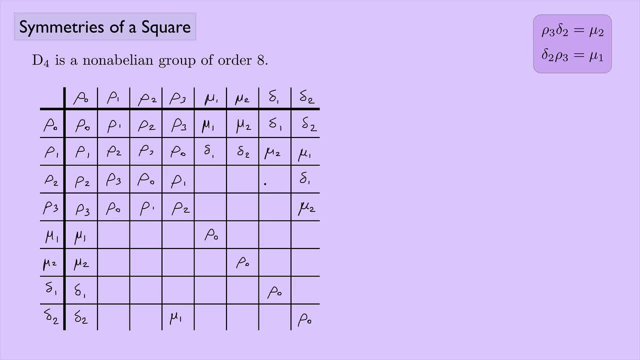 Okay, and I'll give you a few more of these here. Let's see, what else can we do? 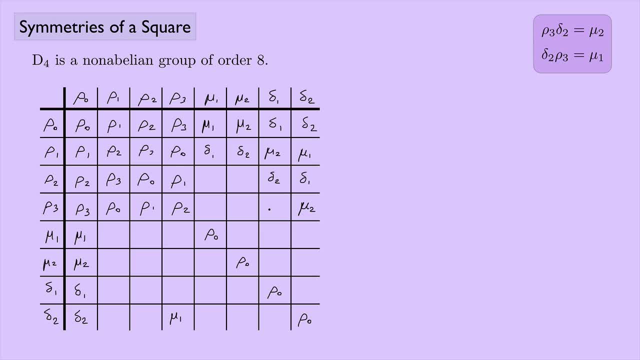 This is a delta 2 right here, and if that's a delta 2, this has to be a mu 1, and this right here is a mu 2, and this is a mu 1, and this is a delta 1, and this is a delta 2. Great. 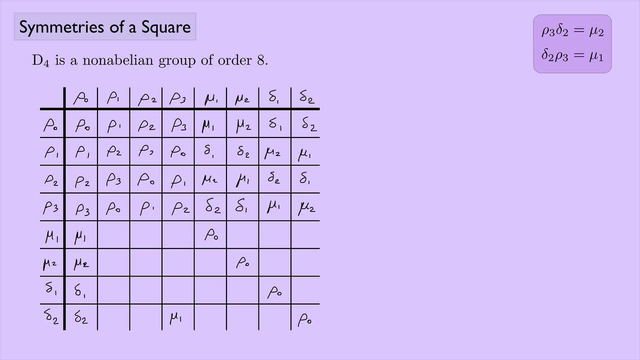 Okay, how about on this side over here? So let's look at this 4 by 4. So we have this row, this column right here. How about these ones along the bottom? 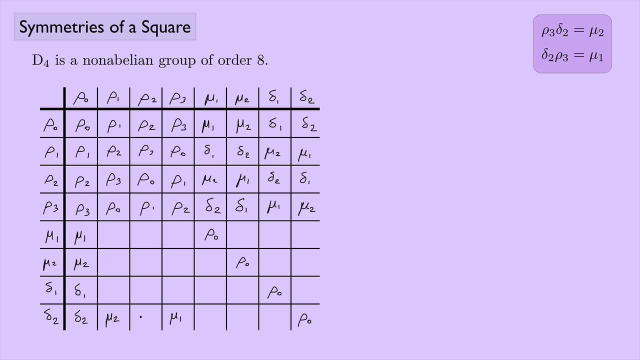 This is a mu 2 right here, and this is a delta 1. All right, and this is a mu 1 right here, and again, I'll leave you to check these computations yourself so you can see that 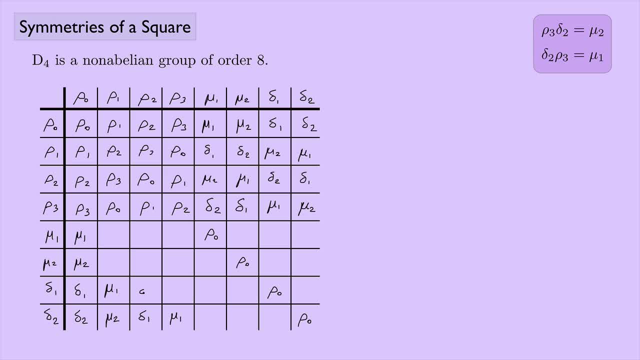 they actually do work, and this is a delta 2 right here, and this is a mu 2 right here, Okay, so now these two have to be deltas, and these two have to be deltas, and so if I know one of them, I know the other three. 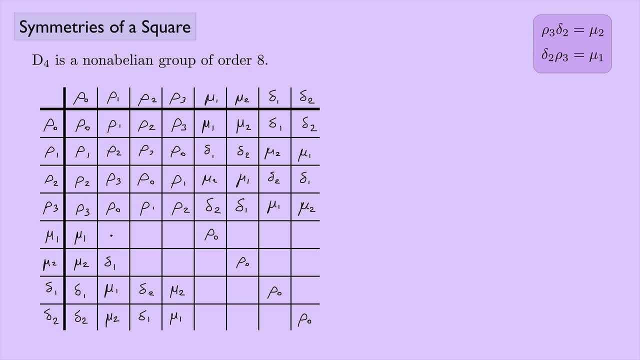 This one right here happens to be delta 1, which means this is delta 2, which means this is delta 1, which means this is delta 2. Great. 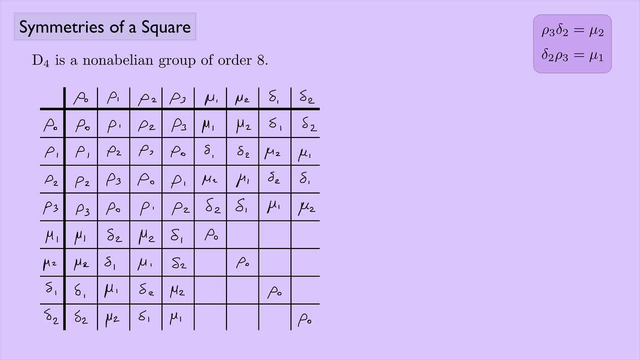 And this has to be mu 1, and this has to be mu 2, because I already have a mu 2 here, so. 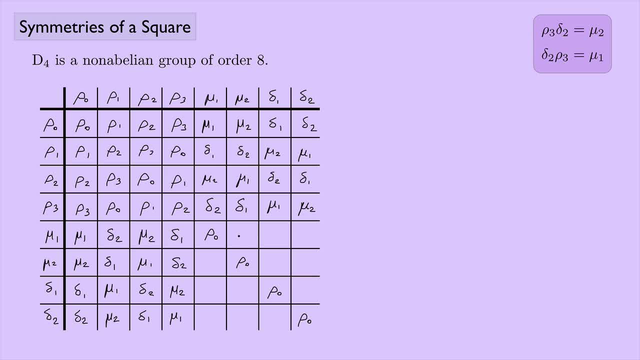 Now I just need to do this part down here, and so I'll tell you that this is a row 2, this is a row 3, and this is a row 1. This is a row 3, and this is a row 2. 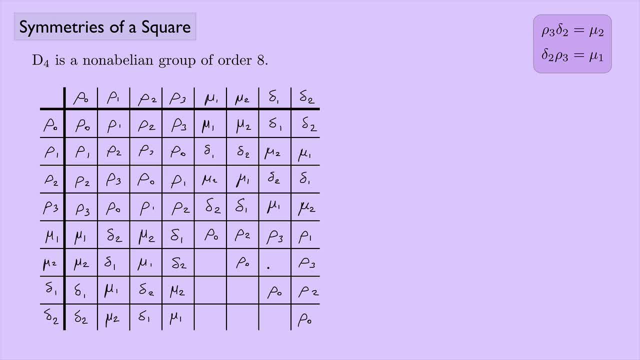 And so let's see, what else can we do based off of this? Well, we must have row 1 and then a row 2, okay? And then we have to have a row 1 somewhere down here. 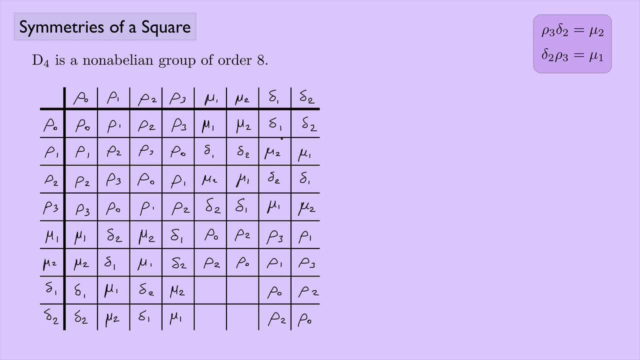 Well, I know right here this has to be row 2, because I don't have a row 2 yet in this column. 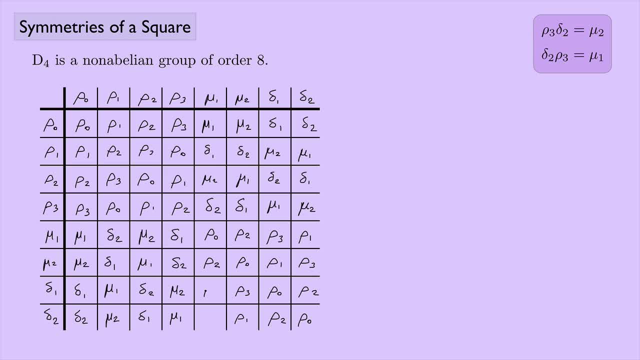 And this is a row 1, this is a row 3, which means this is a row 1, and this is a row 3. 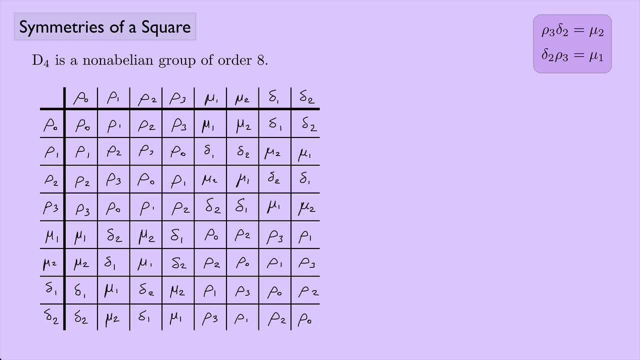 So again, I'll let you check all of the entries in the table, and again, remember that in each row and each column, each element should appear exactly once. 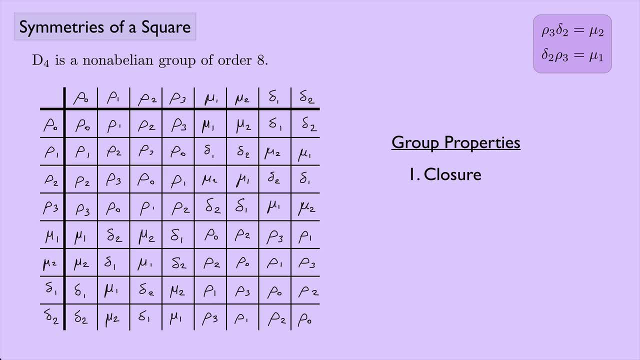 So, is this a group? Well, let's look at the group properties. Is it closed? It is indeed closed. Is it associative? Well, we know that composition of functions is associative, so this is associative. Is there an identity? Well, you might guess that row 0 is the identity, and it is. That's the thing that leaves the square alone. 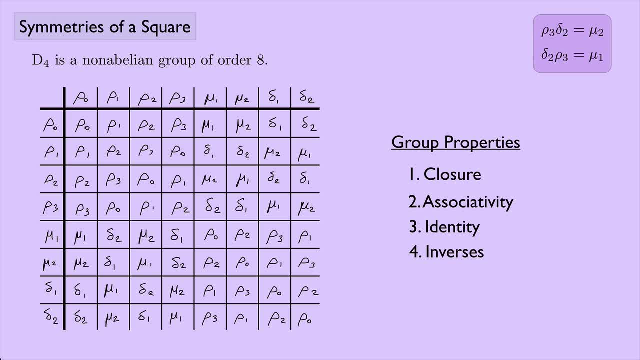 And what about inverses? Well, we see that row 1, if we look at the table right here, row 1 and row 3 are inverses of each other, row 1 and row 3. And row 2 and row 2, let's see, so row 2 is its own inverse. And then all of the flips are their own inverse, all of the mus and the deltas. So yes, everything does have an inverse, which means that this is a group, in fact, it is a non-abelian group, meaning that the operation is not commutative. 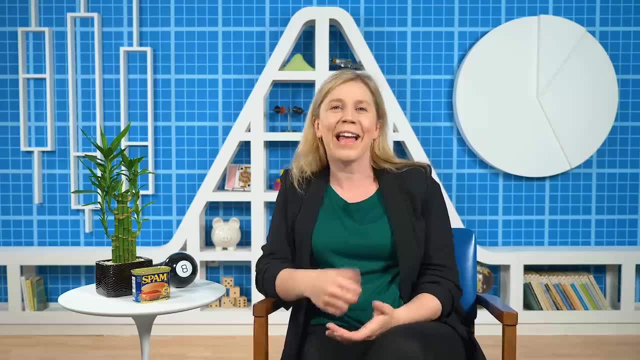 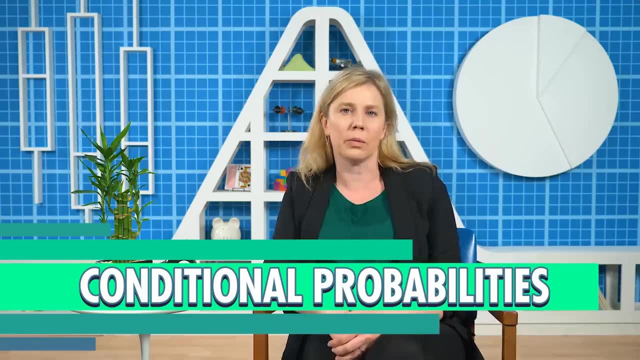 Hi, I'm Adriene Hill and welcome back to Crash Course Statistics. We ended the last episode by talking about conditional probabilities, which help us find the probability of one event given that a second event has already happened. But now I want to give you a better.